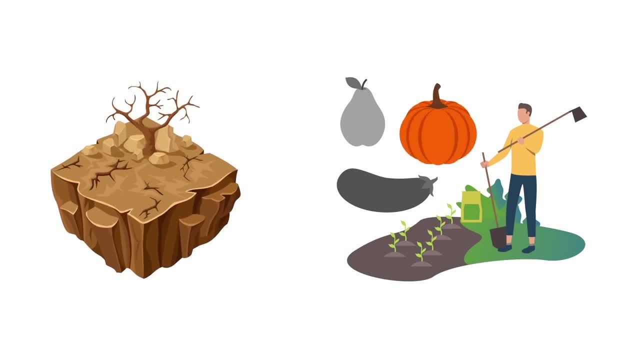 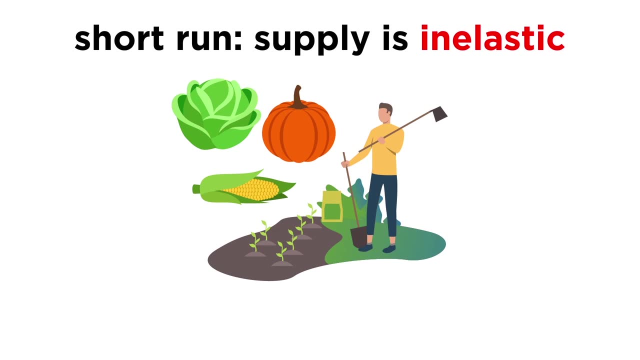 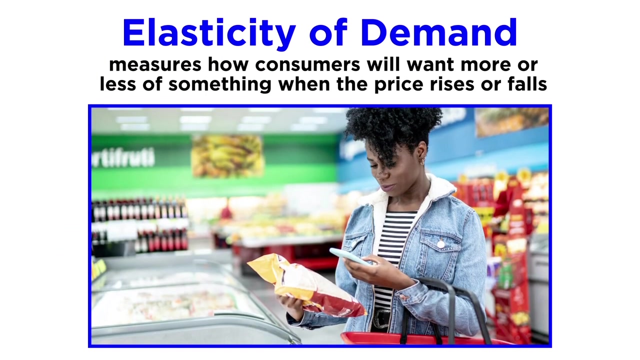 of future droughts, or perhaps the farmer might adjust the types of crops that are planted. Regardless, in this case, in the short run supply is inelastic and in the long run supply is more elastic. Elasticity of demand measures how consumers will. 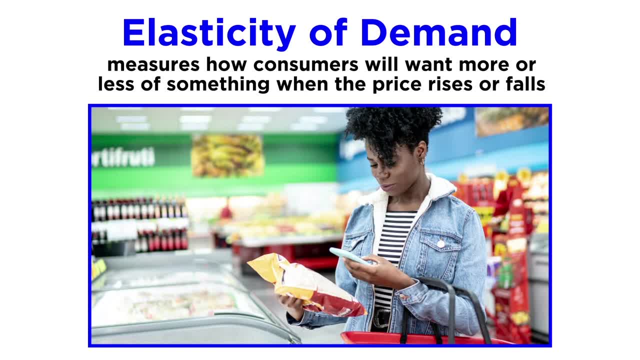 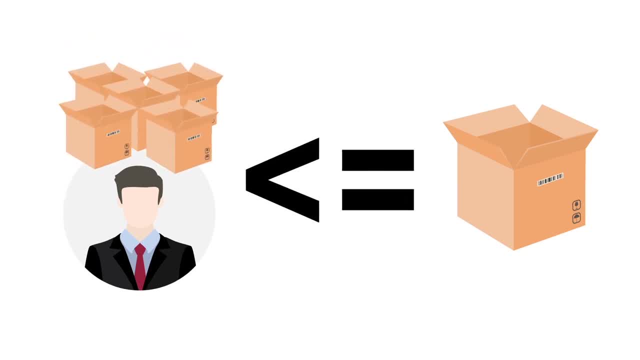 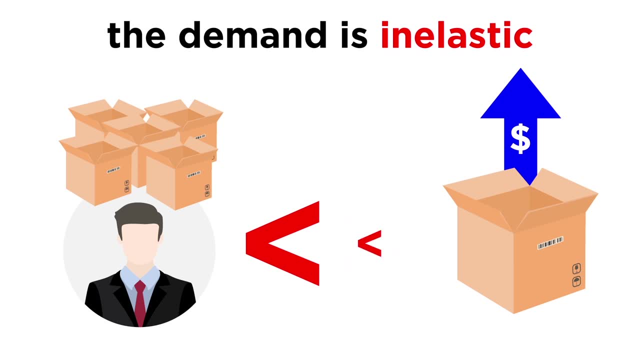 for example, want more or less of something when the price rises or falls. If people buy the same amount or just a little less of a good or service after a large price increase, the demand is inelastic, meaning it doesn't change much If people buy much less of a good or service after. 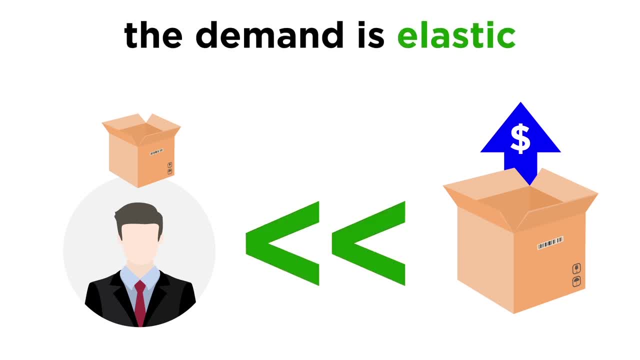 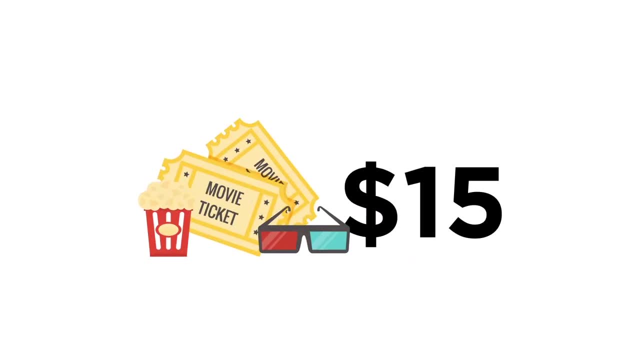 a small price increase. the demand is elastic, meaning it can change a lot. For example, if movie tickets went up from $12 to $15, but you don't care, because you really want to see the latest blockbuster movie on the big screen. 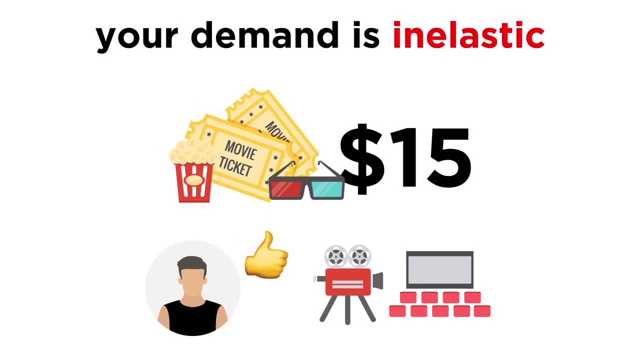 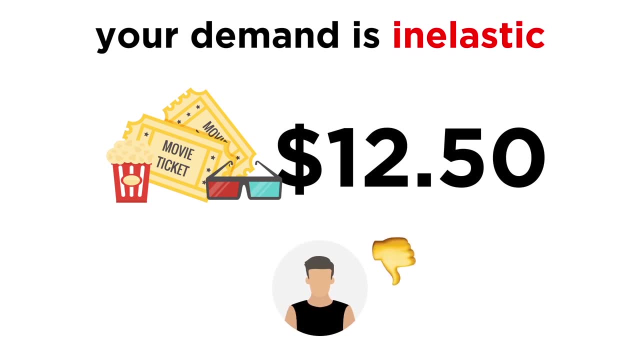 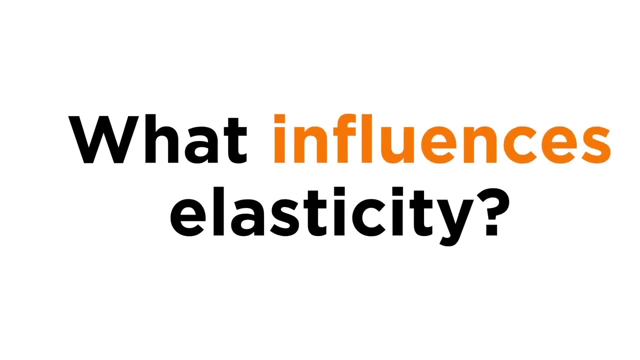 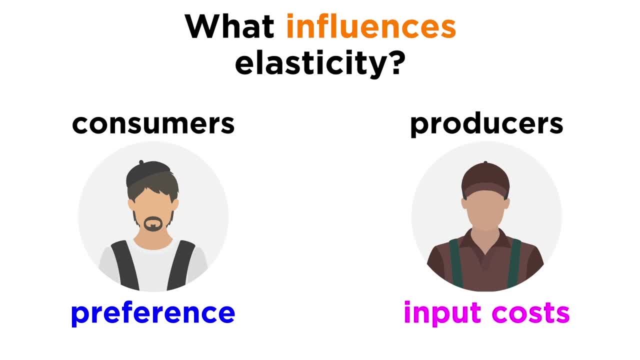 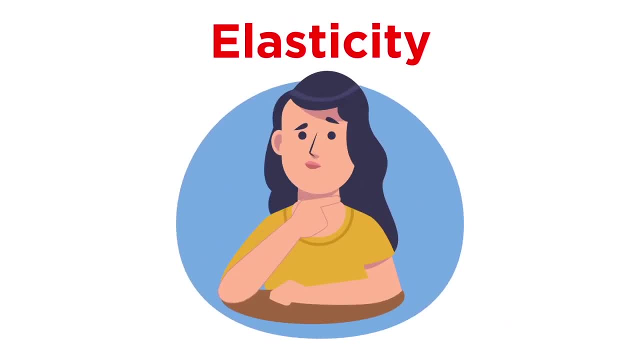 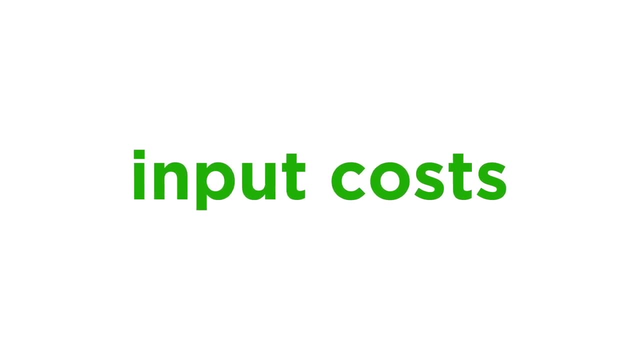 For producers, it comes down to what it costs to produce something. This is also known as input costs. With elasticity understood, let's focus on changes in supply First. let's stay with the influence of input costs. Often, input costs can drop due to advances. 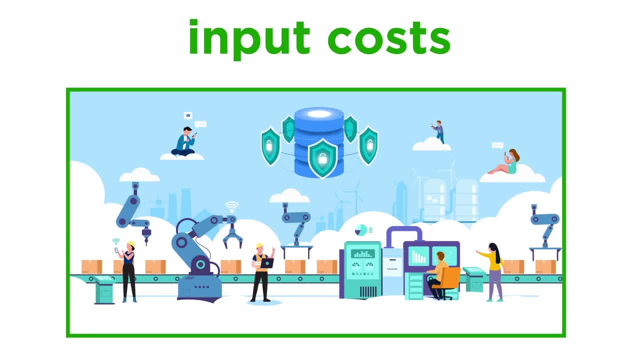 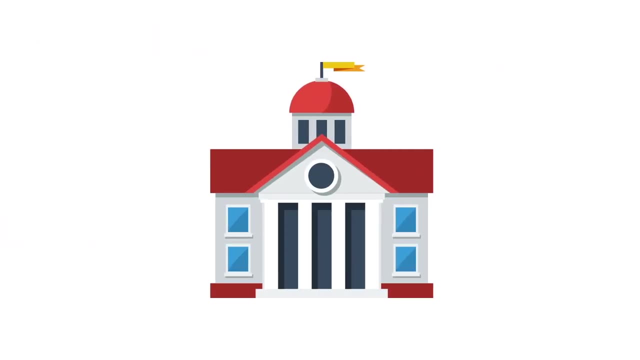 in technology. Automation, including the use of artificial intelligence and robots, has made the manufacturing process more efficient, thus saving on labor costs. Because of this, producers can produce more for less money. Government policies can also change the supply of a good or service in both a positive and negative way. For example, a government can 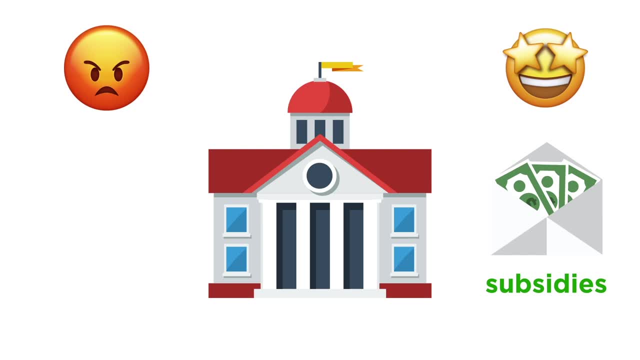 provide subsidies. A subsidy is essentially money from the government intended to give a boost to certain businesses or industries. Conversely, governments can also establish excise taxes, meaning taxes on the production or sale of a good which reduce production. Other supply determinants or influences which affect supply. 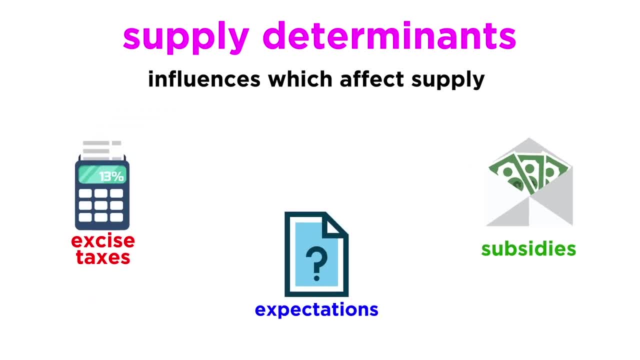 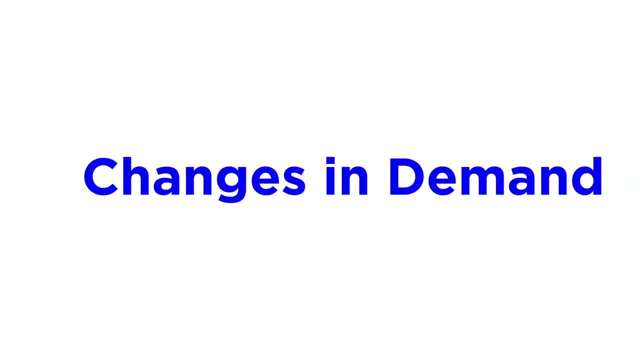 include expectations about what a price might be and the number of competitors also producing the same good or service. Next, let's examine changes in demand, Assuming all other factors don't change. here are the following factors. First, let's look at the number of competitors. 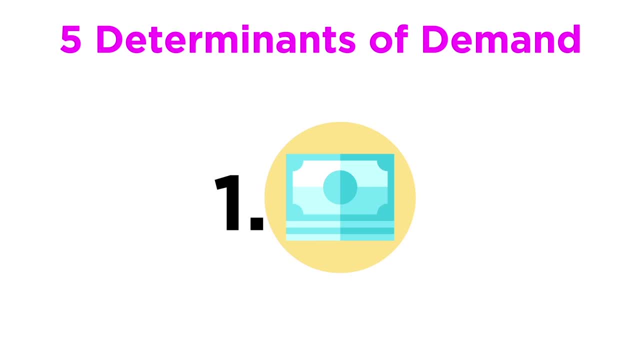 Here are the five determinants of demand. Number one: changes in a consumer's income. The more money consumers make, the more they will demand goods and services, and the less money they make, the less they will demand goods and services. Number two: consumer expectations, Our expectations. 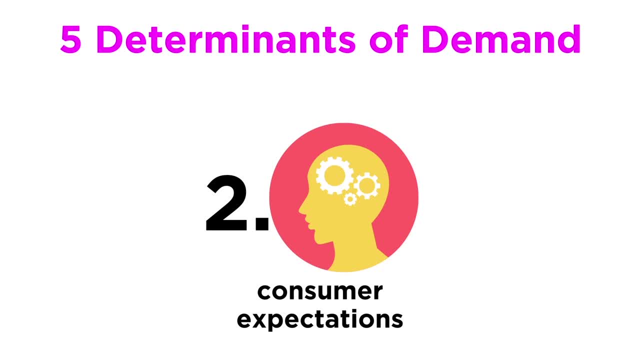 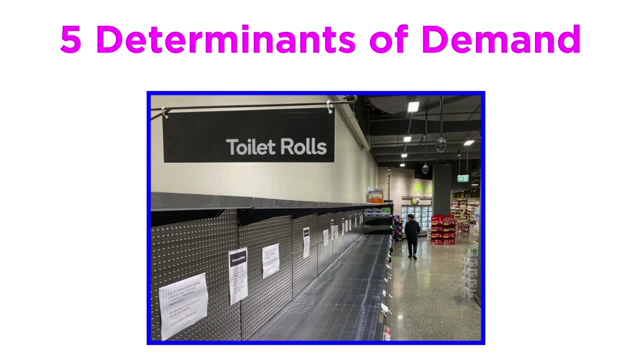 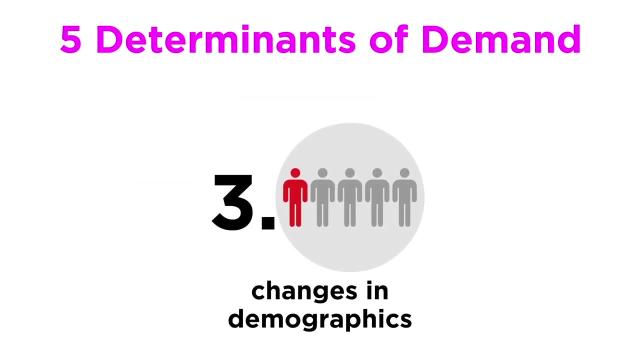 whether they are hopes or concerns, can affect our demand for certain goods and services today. For example, an expectation that there will be a shortage in a particular product may influence consumers to buy more of it now. Number three: changes in demographics and 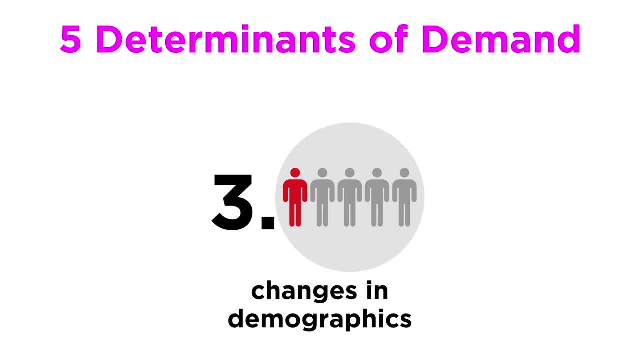 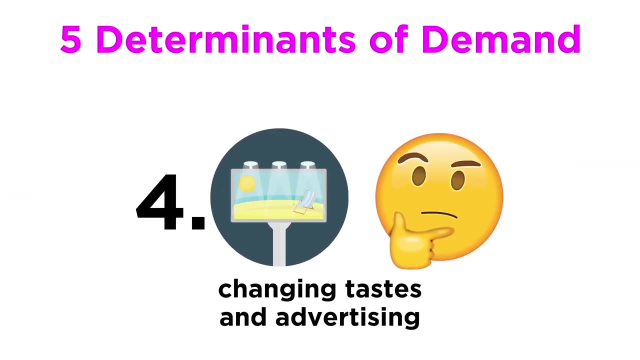 population size can also affect demand. For example, if a real estate developer wants to invest in Texas, they have to look at the growing Hispanic American population there to have a better prediction of what demand will specifically look like. Number four: changing tastes and advertising, Keeping up with social trends and 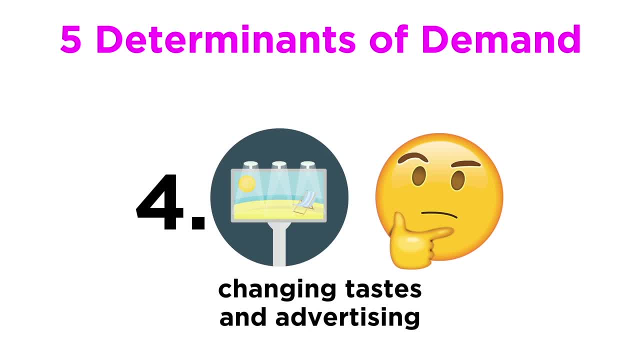 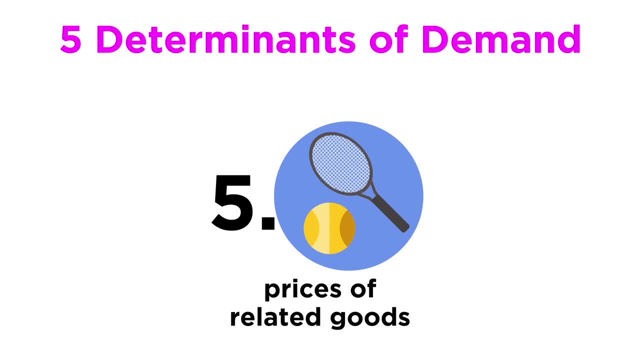 general preferences help predict what demand will look like. And finally, number five prices of related goods. Demand can simply shift in response to a change in the demand for another related good. There are two types of related goods that interact in this way. 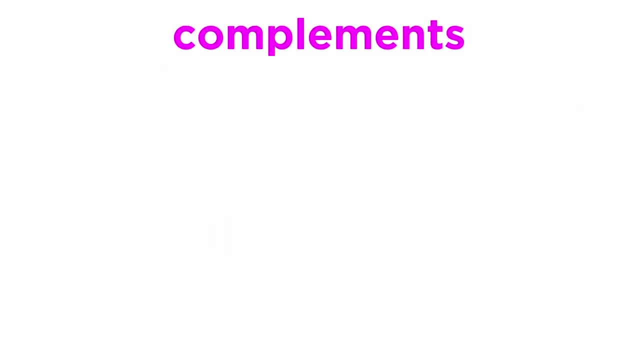 complements and substitutes. Complements are two goods that are bought and used together. They complement each other, hence the name. When we consider the demand for tennis rackets, tennis balls are considered a complement, since playing tennis requires both items. Substitutes are goods that are used in place of one another. They substitute for each.